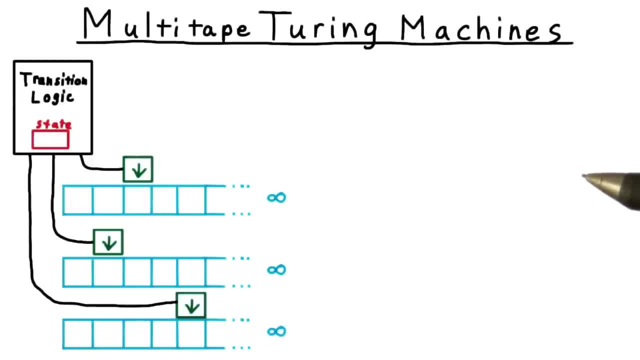 Since having multiple tapes makes programming with Turing machines more convenient and since it provides a nice intermediate step for getting into more complicated models, we'll look at this Turing machine variant in some detail. As shown in the figure here, each tape has its own head. 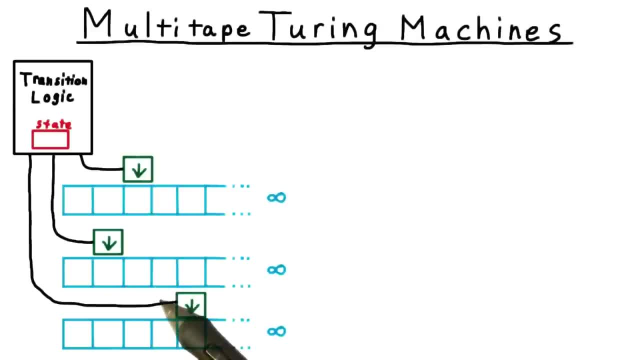 and what the Turing machine does at each step is determined solely by its current state and the symbols under these heads. At each step it can change the symbol under the heads and move each head to the right or the left, or just keep it where it is. 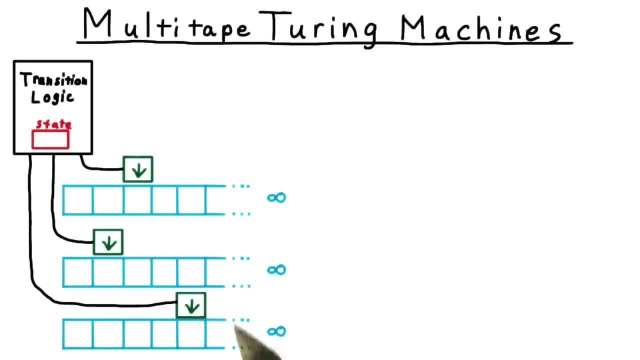 With a one-tape machine, we always force the head to move, but if we required that condition for multi-tape machines, the differences in head positions would always be even, which leads to awkwardness in programming, so it's better to allow the heads to stay put. 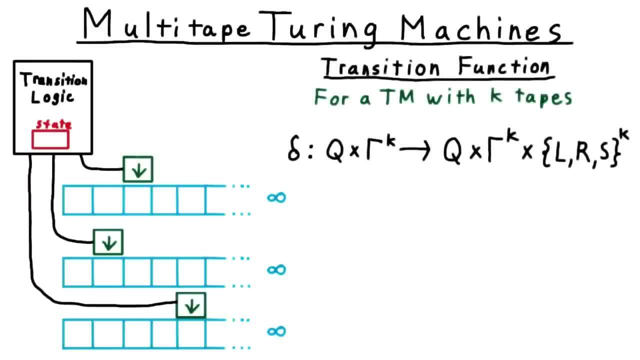 Except for those differences, multi-tape Turing machines are the same as single-tape ones. We only need to redefine the transition function. For a machine with k tapes, the new transition function is from the Cartesian product of the possible states of the machine. 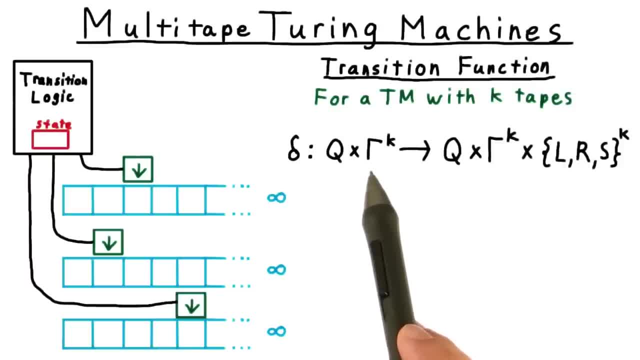 and the possible symbols under the tape. heads to the new states of the machine. times the symbols to write under the heads times the possible directions to move the heads. Everything else stays the same. 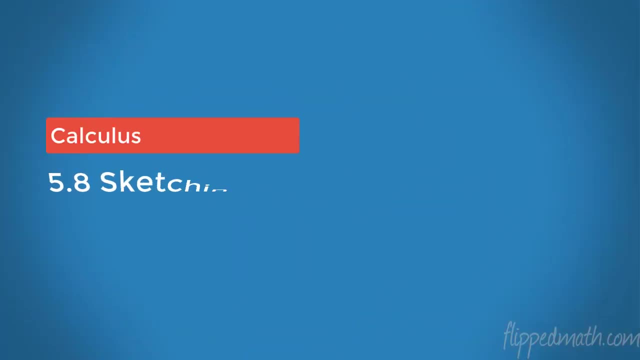 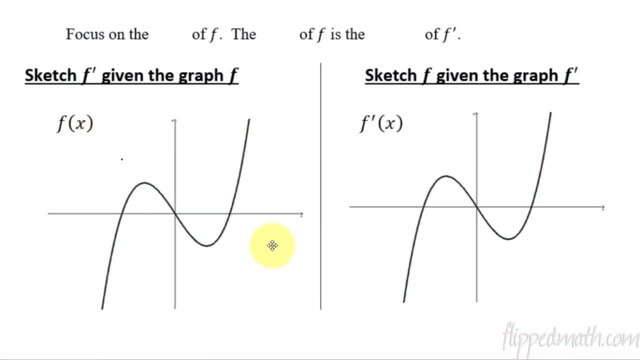 Hello there, calculus kids. This is Mr Bean. Welcome back to another lesson in calculus, and today we're going to talk about how to sketch some graphs from the derivatives and functions, how they intermix with their graphing. Now, this is actually gonna be a pretty short lesson, but just because it's short, and easy to. 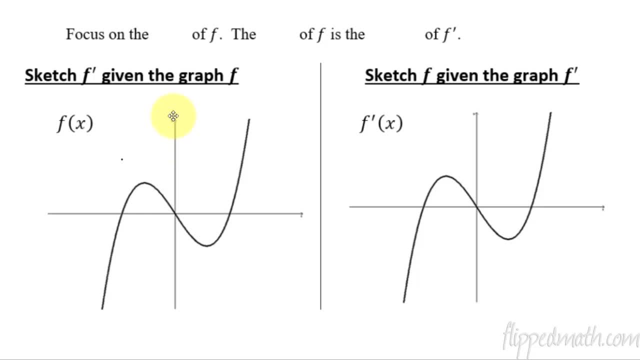 explain doesn't necessarily mean it's easy to understand. So the packet is just a little bit longer. because there's several practice problems on these, this material, because this stuff is all over an AP exam. You've got to know how to do this forwards and backwards, So let's focus on the slope of F. Now we know the.